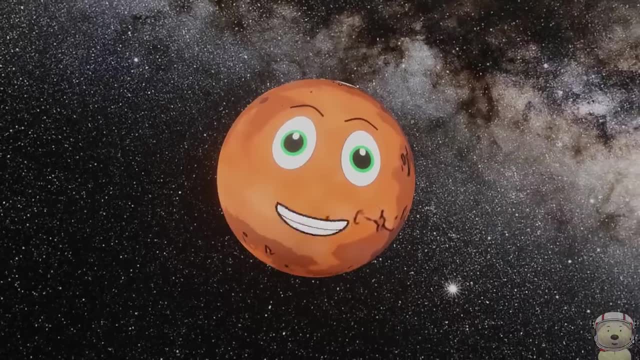 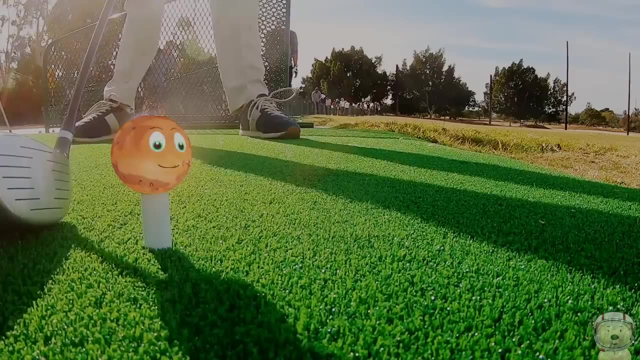 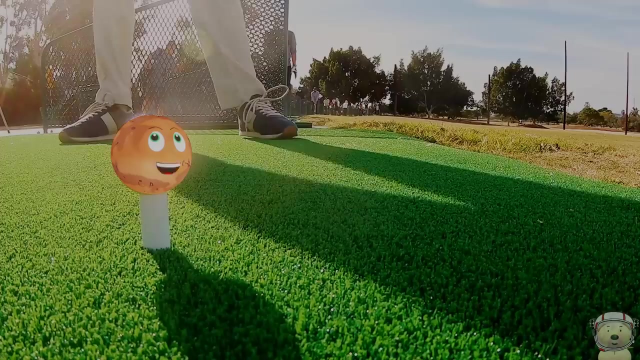 Uh, nothing. If Mercury was a ping pong ball, I suppose you could compare me to a golf ball. Uh, hang on, I'm not sure I like the sound of this now. Uh, wait, what are you doing? Whoa. 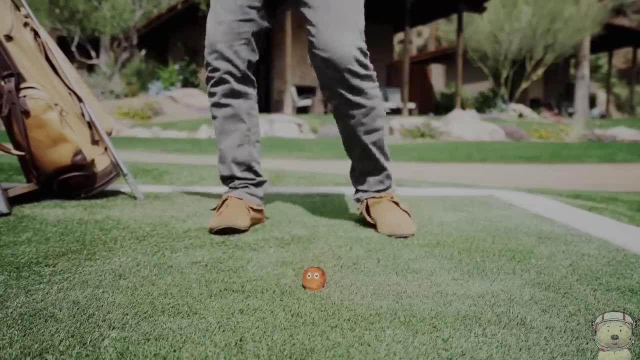 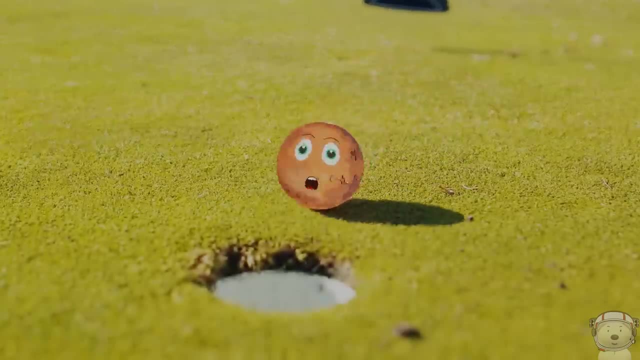 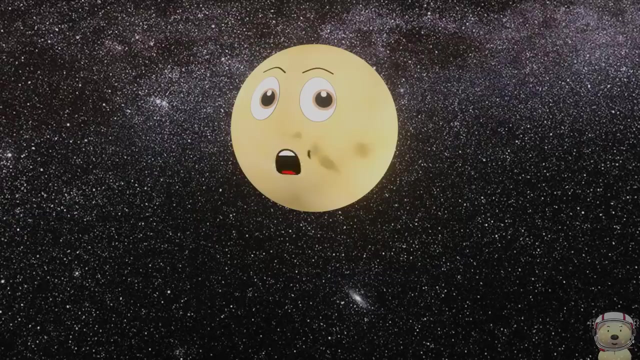 Uh, um, hang on. Whoa, whoa, whoa, whoa, whoa, whoa, whoa. I'm busy. Next up me, planet Venus. As we all know, I am fabulous. If Mars was a golf ball, I would be a tennis ball. 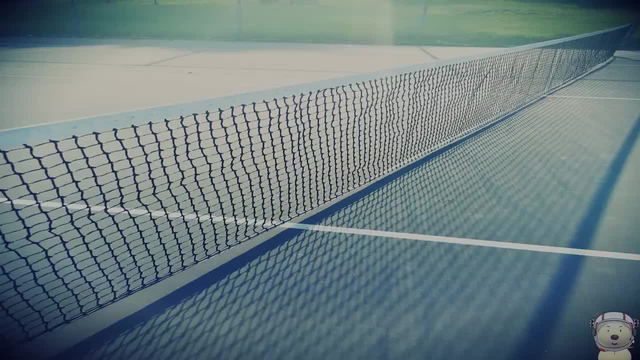 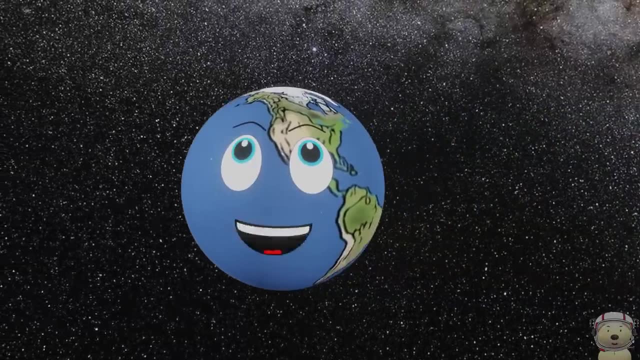 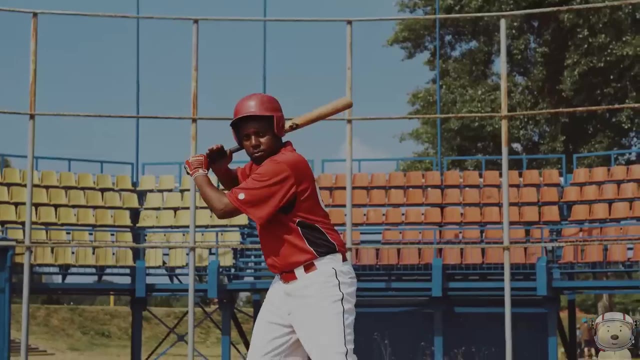 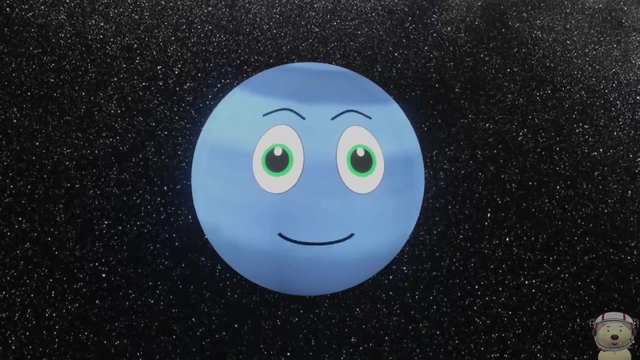 Whoa, Whoa. Now it is me, planet Earth. If I was a sports ball, I would be a baseball Similar in size to Venus, But not as fabulous. Anyway, Whoa, Now it is me, planet Neptune. 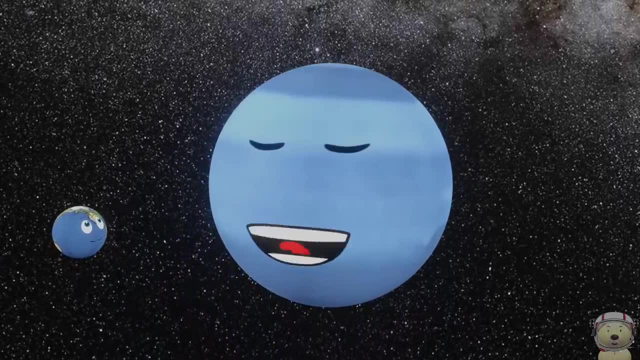 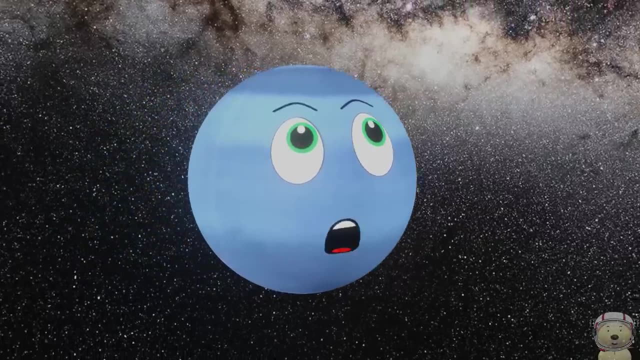 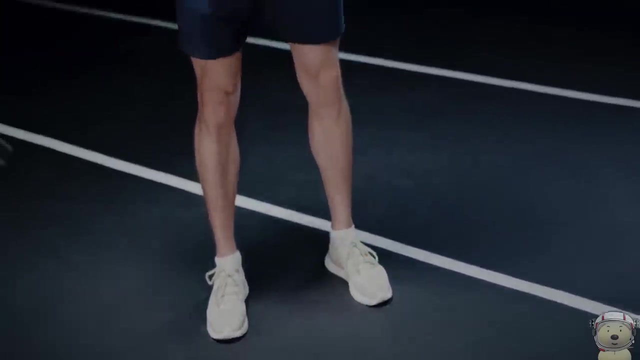 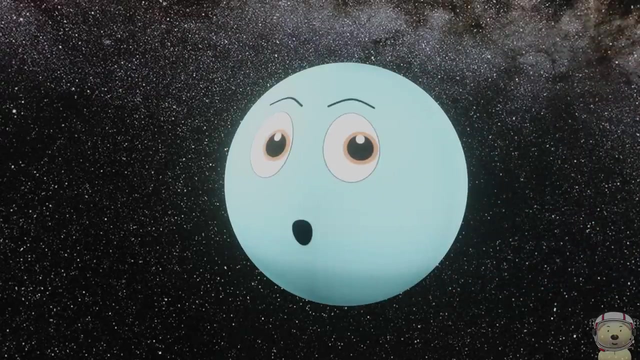 Hey Neptune. As you know, I am the windiest planet in the solar system. Whoa, But if I was a sports ball, I would be most like a volleyball. Whoa. Hey you, It is me, planet Uranus. 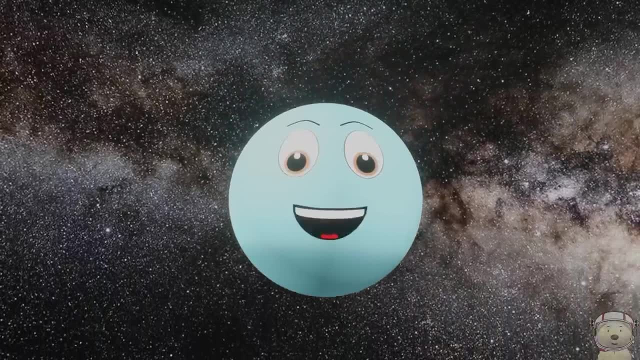 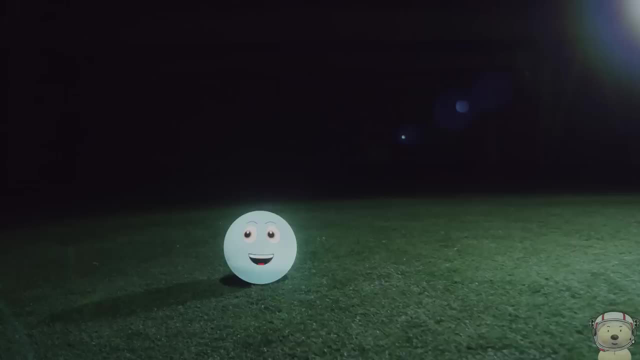 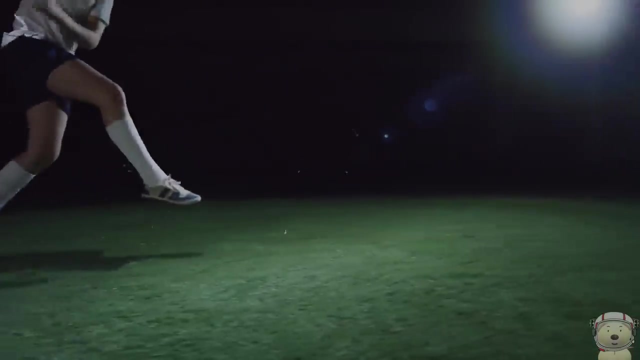 If Neptune was a volleyball, I would be a football. That is a soccer ball. Wait, How did they hit a football With their- what? Their feet, Oh dear, Whoa, Whoa, Whoa, Whoa, Whoa. 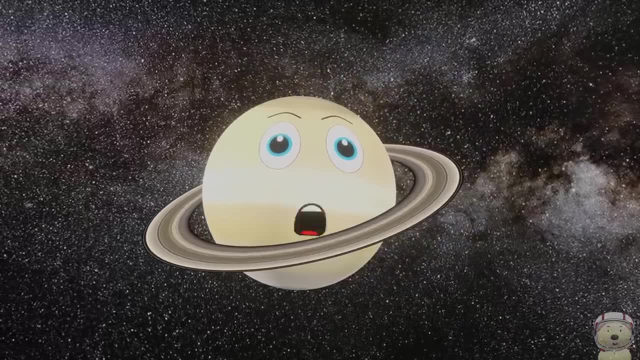 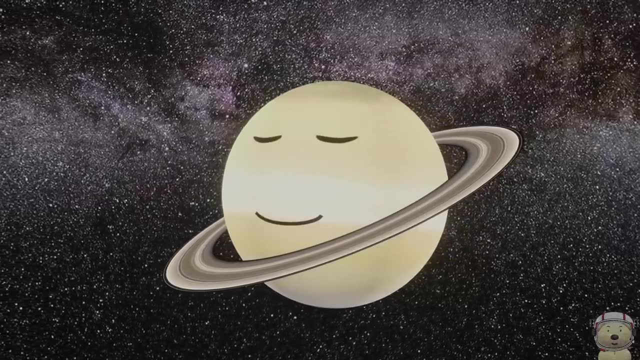 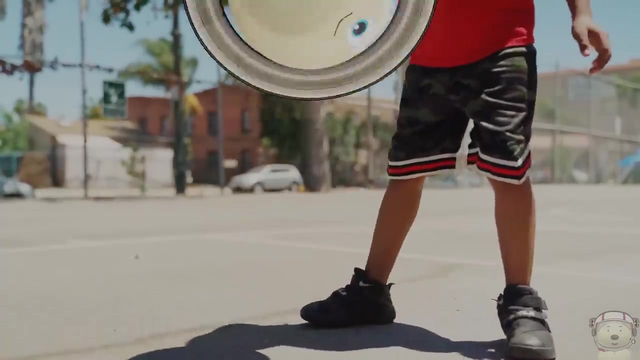 Now, dudes, If Uranus was a football, Whoa, There is no ball big enough for me, But the nearest would be a basketball. Oh yeah, Oh yeah, Oh yeah. Plus, I have my own hoop too.